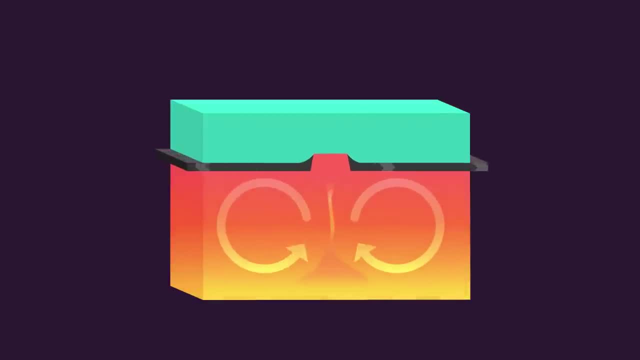 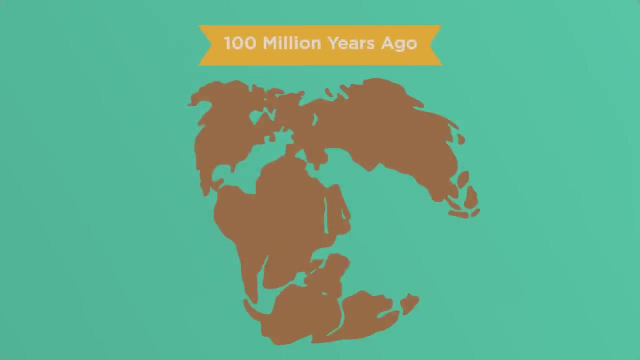 plates move apart and new magma, which is molten rock, erupts to fill the gap, forming new oceanic crusts made of basalt and igneous rock, and this is called a divergent boundary. A hundred million years ago, when dinosaurs roamed the earth, Europe and America were joined and there was no Atlantic. 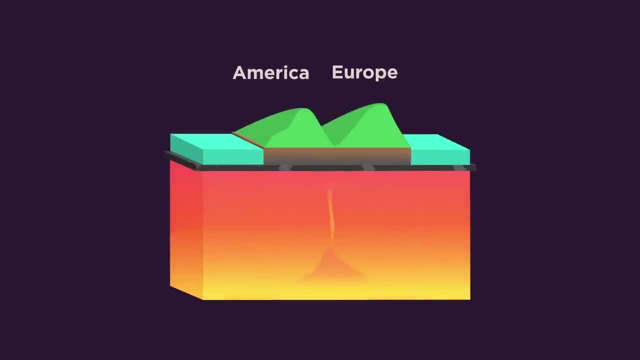 Ocean. These convection currents gradually pulled the two continents apart. The plates move apart and the ocean is formed. First, a rift valley formed which got flooded with seawater, and the new Atlantic Ocean was born. Even today, the Atlantic is spreading about as fast as your. 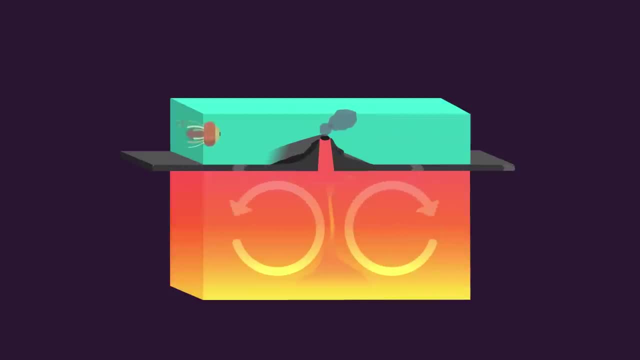 fingernails grow, and down the middle are underwater volcanoes where strange life forms grow amongst the so-called black smokers. If the ocean is spreading in some places, it must be being consumed in others, and this is where two plates are moving towards the ocean and the ocean is moving towards. 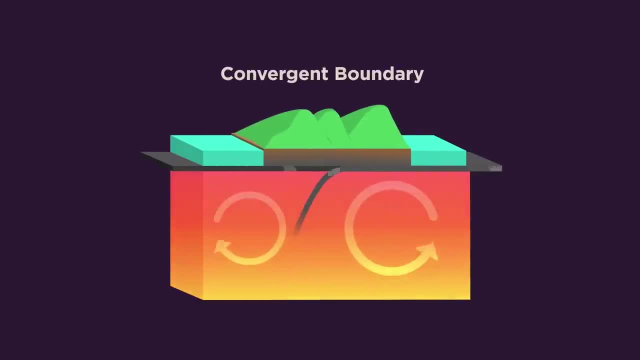 the ocean, and the ocean is spreading in some places, it must be being consumed in others, and this is where two plates are moving towards each other, the so-called convergent boundaries. Continental rocks get eroded and form a sediment on the ocean floor As the ocean crust is carried down, called subduction, the sediments get carried. 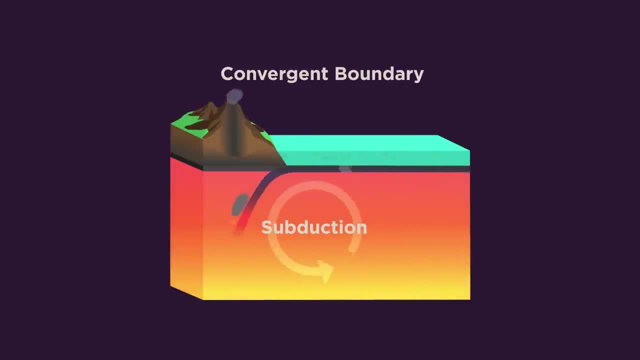 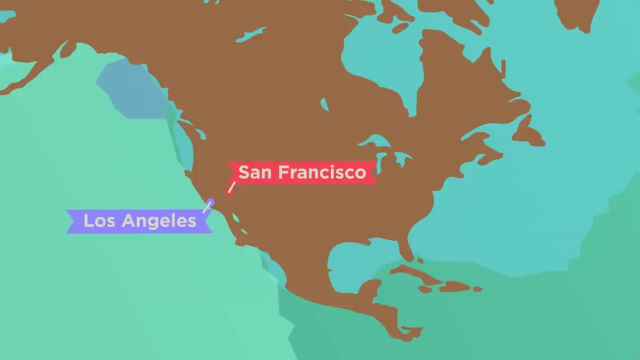 down or subducted and melt, but, being less dense than the basalt rock of the ocean crust, get pushed up, forming volcanoes along the mountain chain. Sometimes the plates simply slide alongside each other, as they do in the famous San Andreas Fault in California. The relative 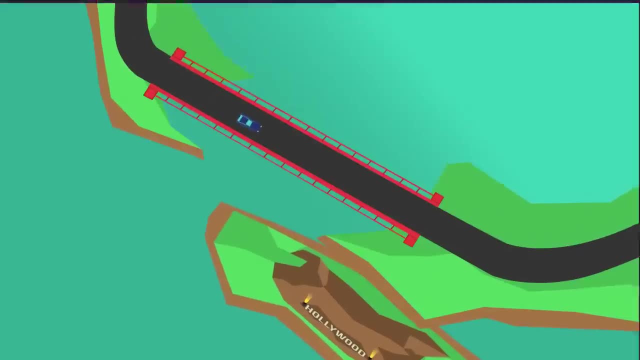 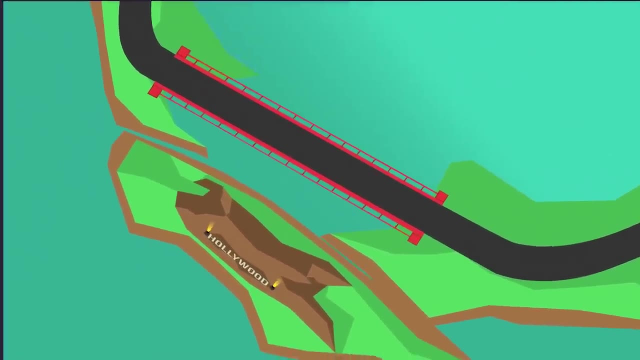 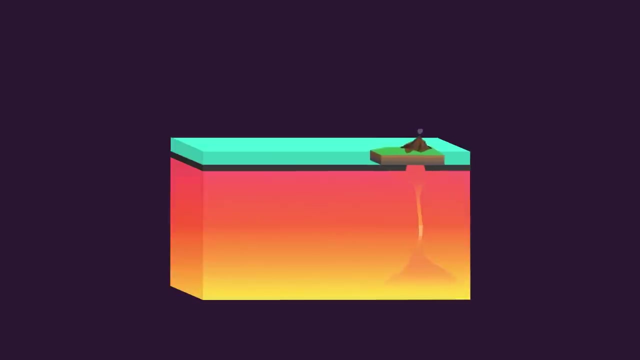 movements in the so-called transform boundary cause major earthquakes. It will also mean that Los Angeles will come alongside San Francisco in about 20 million years time. Sometimes a convection current in the mantle is just a single upwelling, causing what is called a hotspot As the plate. moves over this hotspot, the sediments get eroded and melt, but, being less dense than the basalt rock, a series of islands form, as we see in Hawaii. Gradually, the older islands get eroded and disappear beneath the ocean. Oceanic crust is never more than a few hundred million years old. 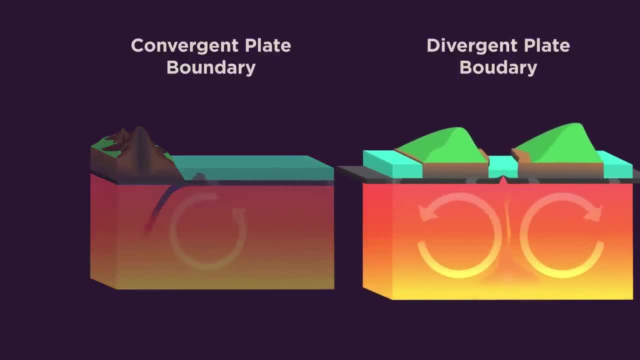 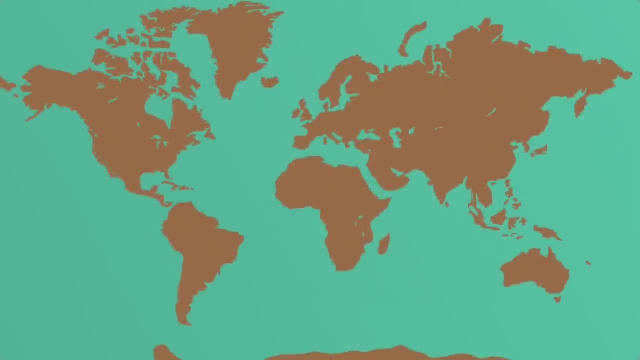 because it is constantly being created at mid-oceanic ridges and consumed or subducted. at convergent boundaries. However, continental crust has simply been carried around, broken apart and brought together in the middle of the ocean to form a sediment. The sediment has been in the ocean ever since it formed the earth 4.5 thousand million years ago.